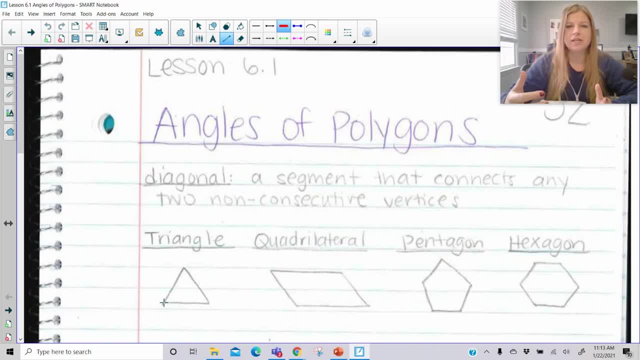 another they're touching. It's a side That's not considered a diagonal, So a triangle has no diagonals in it. A quadrilateral is a segment that connects any two non-consecutive vertices. I can take a vertex here and connect it to this opposite point. And whoa, that was just too much. 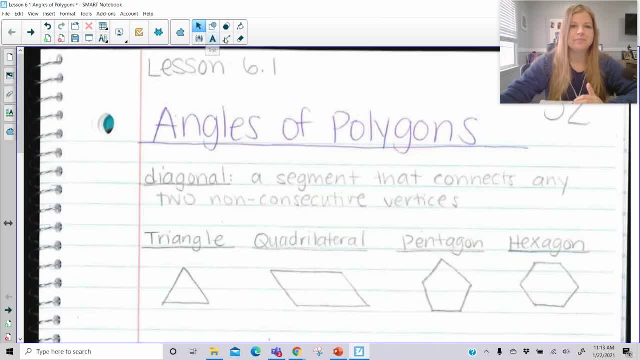 So I'm going to redo that line. Too much, too much, And so this is a diagonal. It's connecting one vertex to another vertex that's not consecutive, And if I connected it to, let's say, this point here, that would be on the side And we just don't want that. I can have another diagonal. 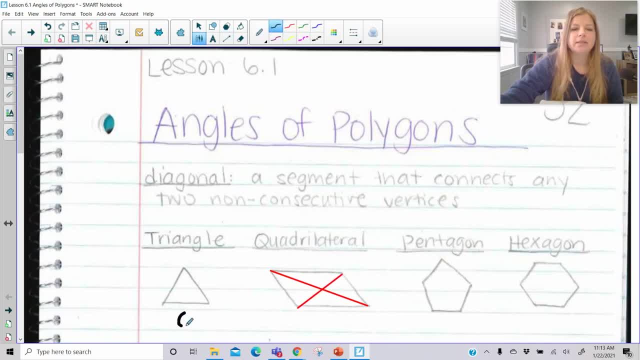 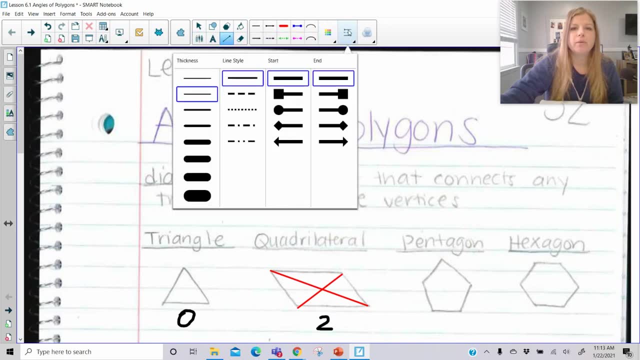 So a triangle So far has zero diagonals. A quadrilateral, a four-sided figure, has two. So now let me go over and try out a pentagon. So I'm going to start from the top point, It doesn't matter what point. 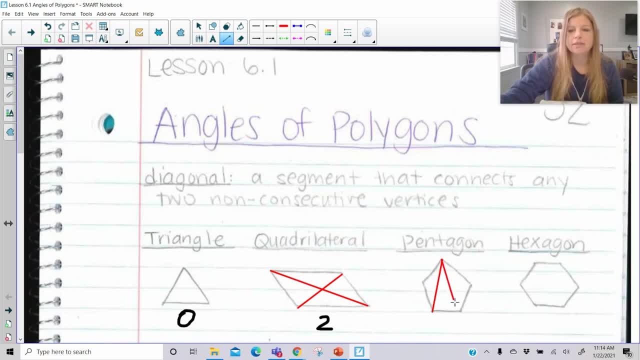 you start with, And here I can connect it twice and create two diagonals From this point. here I can extend it. So what I'm trying to do is I'm trying to create as many unique diagonals as I can, And when I do that, what you'll notice is the amount of diagonals I was able to make. 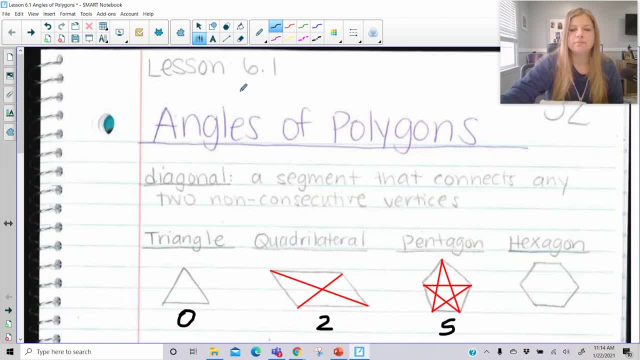 is five, It's a star And a hexagon. So if I start, let's say, from this point, here I can make one, two, three, then four, five, six, seven, eight, nine. So in a hexagon I can make nine diagonals. Something we might notice about patterning here: 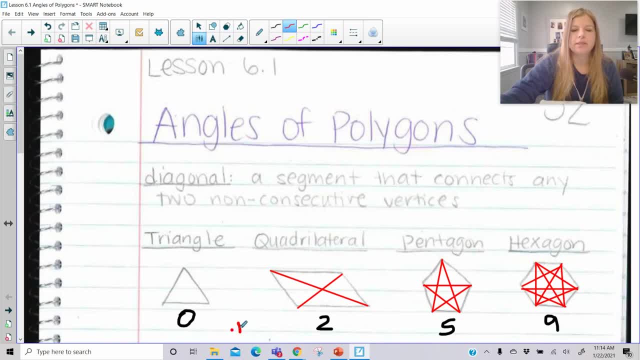 from zero to five. nine is, you might say, okay. well, look, it's increasing by two And then it's increasing by four And it's increasing by. I'm sorry, why did I put four there? I'm just having a bad day. I'm not going to edit this out. either Three and then four. 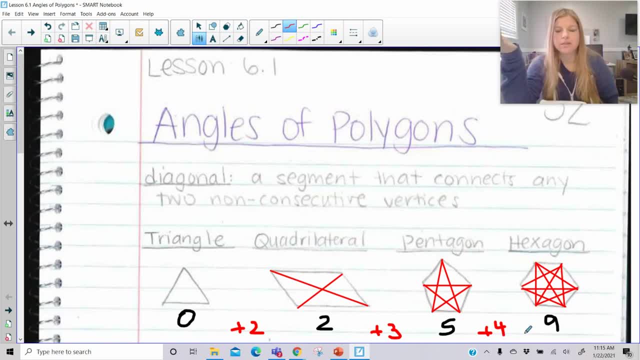 So, as the number of sides increases, I can make nine diagonals. So I can make nine diagonals. The number of diagonals is increasing, adding on to the previous amount by one more. So adding two, adding three, adding four. the next one that we could then say is going to add by five. 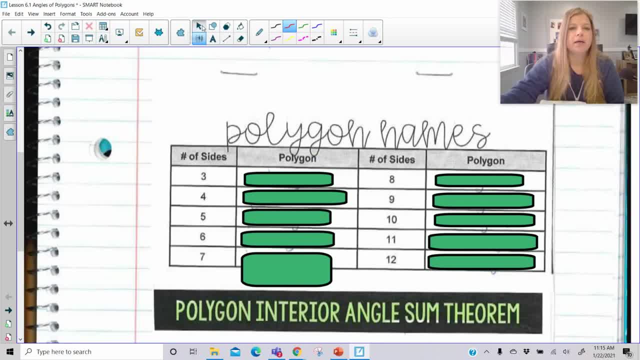 Polygon names. So these are going to be some classic polygon sides- number of sides rather- and the names that go along with those polygons. So we should know a three-sided figure is a triangle, A four-sided polygon sometimes people want to say square or rectangle. 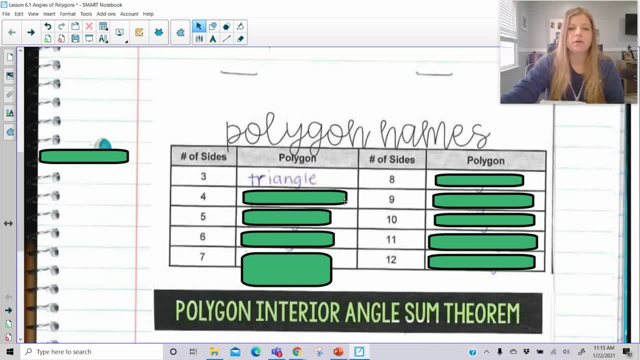 but that's a specific polygon. So a four-sided polygon is a triangle. sometimes people want to say square or rectangle, but that's a specific type of quadrilateral. So when we talk about a four-sided figure we use quadrilateral, because that's the overall name for a four-sided figure. 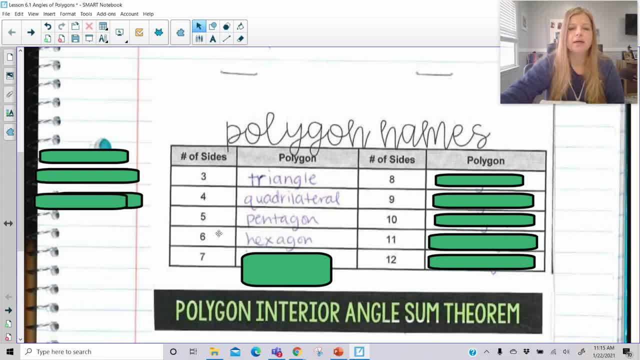 Five side is pentagon, Six side is hexagon. Seven sided is heptagon or septagon. You can see either spelling online, if you were searching something up for a seven-sided figure: Eight is octagon, Nine is nonagon, Ten is dectagon, Eleven is hentagon. 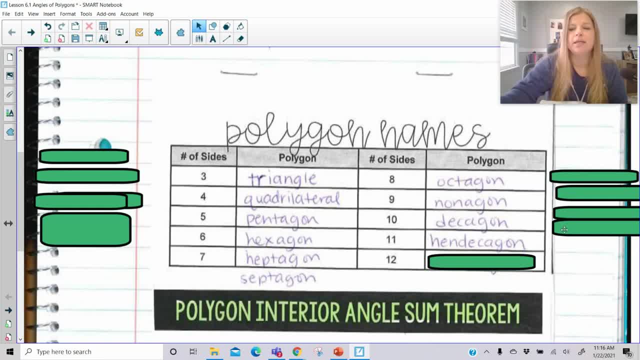 We don't often use 11-sided figure, but that is the name of it, And 12 is dodecagon. And really what happens past 12,? if I say a 13-sided polygon, we just call it a 13-gon, So we put the number of. 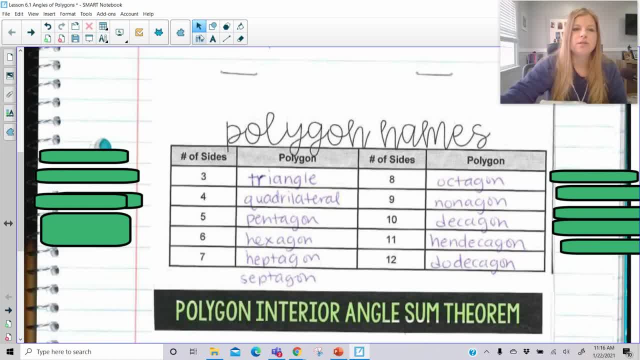 sides dash G-O-N at the end. Something also cool to kind of see here is, if you recall learning in a history class, anything like that, there used to be 10 months in the year, And so the seventh month was September. And so the seventh month was September, And so the seventh month was September. 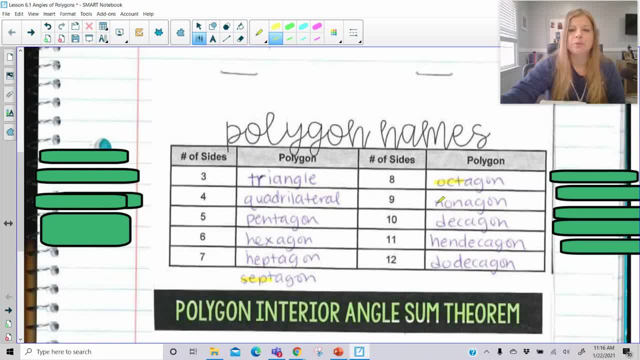 The eighth month was October, The ninth month was November And the 10th month was December, And then they brought in July and August, after the fact, Julius Caesar, Augustus Caesar, to make it 12 months, But that's why you see these prefixes, which is pretty cool. 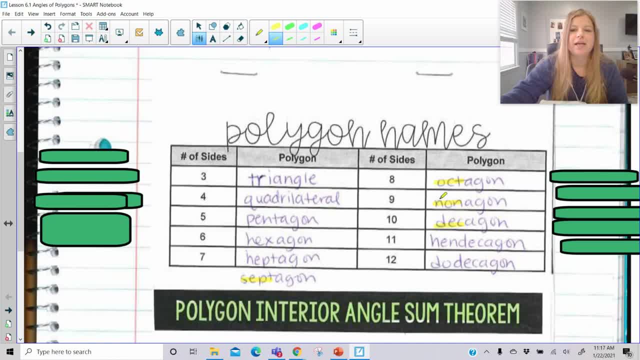 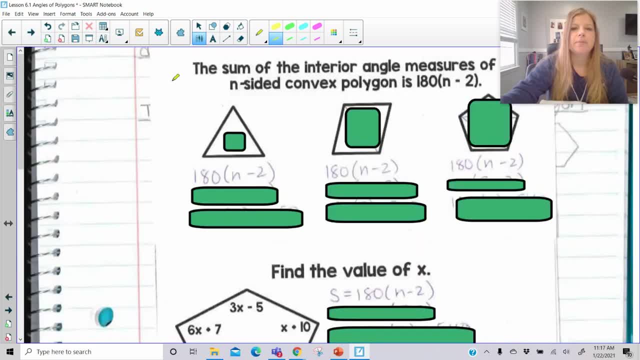 of sept, oct. non and des for seven, eight, nine and 10.. So now, what I want to show you is the polygon interior angle sum theorem. So the polygon interior angle sum theorem is that the sum of the interior angle measures of an N-sided convex polygon is 180 times N minus two. 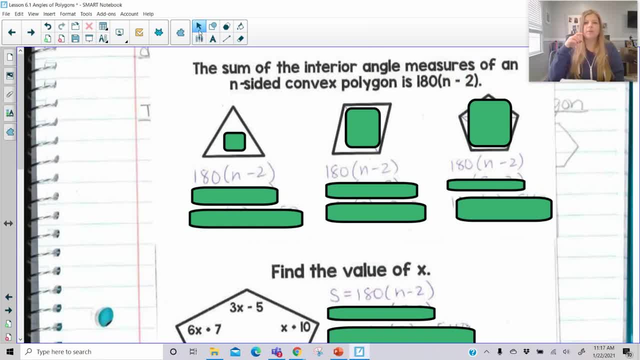 Now here is what this is saying. It's saying: if I want to figure out the sum of all of the interior angles of any polygon, no matter how many sides it has, I'm going to follow this formula. I'm going to do 180 times the number of sides it has subtracted by two. So, really, what I'm doing is: 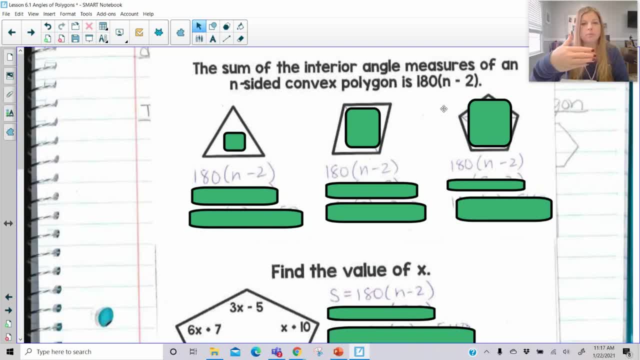 I'm going to take the number of sides, subtract it by two, multiply that result by 180.. So if I gave you a triangle and I go ahead and I substitute in the fact that it's got three sides, well, three minus two is one, and 180 times one is just 180. But we knew that, We knew there's. 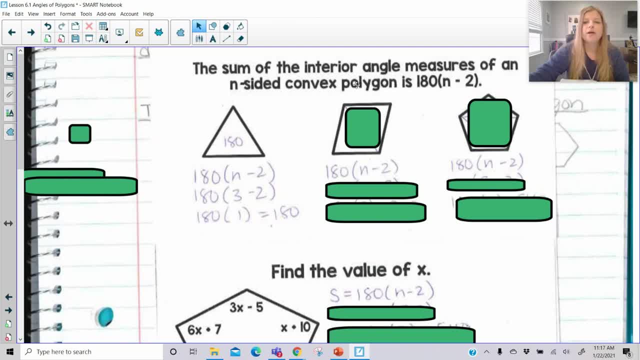 180 degrees in a triangle. If I go over to this quadrilateral here and I go ahead and I substitute in: okay, well, N is now four. I'm doing 180 times two, which is 360.. And most of us should. 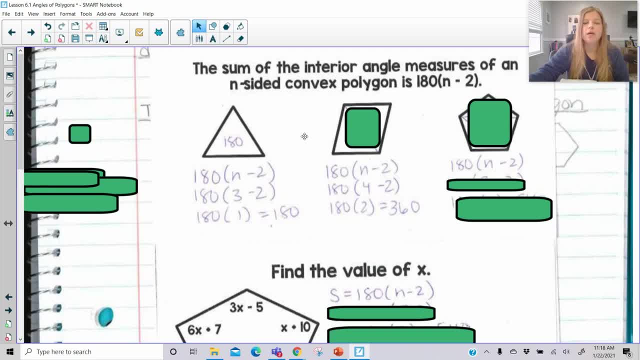 already know, at this point there are 360 degrees in a quadrilateral. So if I go over to this quadrilateral and something that's pretty cool I want to show you is that if you create the minimum number of diagonals, you can actually create 280 degree triangles, and 180 plus 180 is 360. And basically, 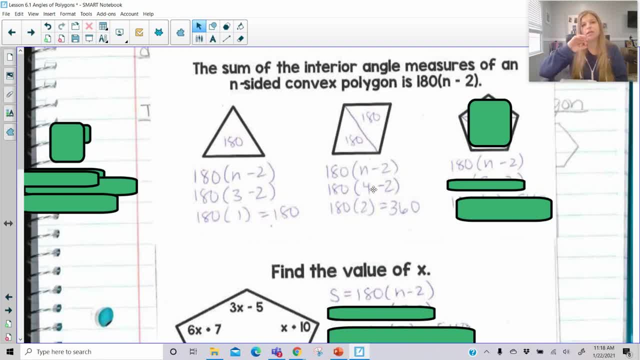 what I mean by the minimum number of diagonals is if you take any vertex and you draw the minimum number of diagonals you can make- or the maximum, really, however many you can- that's going to divide up your polygon into triangles and each triangle is worth 180.. So if I go over to this, 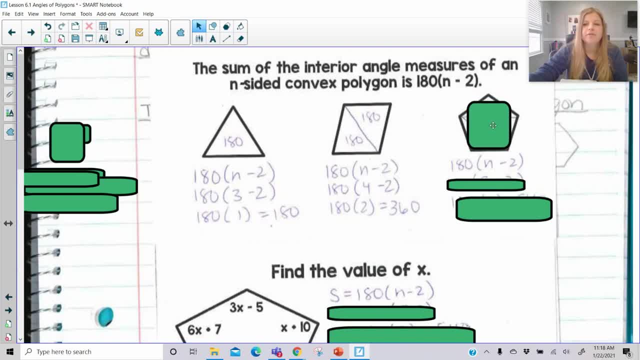 quadrilateral here and I go ahead and I substitute in a five for N and I do: five minus two is three. I end up getting that there's 540 degrees in a pentagon. which? look, if I take a vertex of the pentagon and I draw the diagonals one, two, just the two unique diagonals it's divided up into. 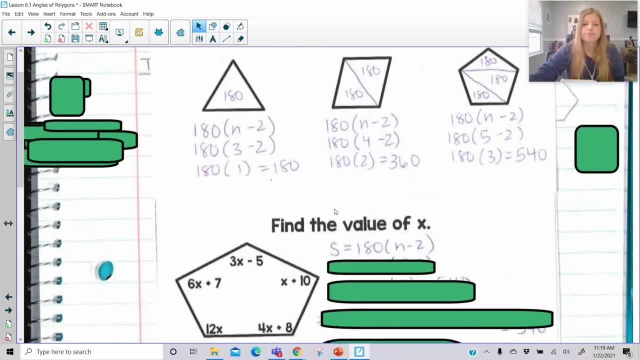 three triangles, which three times 180, is that 540.. If I give you a pentagon and I ask you to find the value of the pentagon, I'm going to give you a pentagon and I ask you to find the value of. 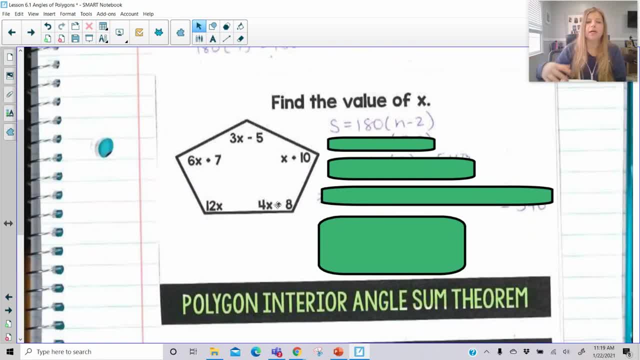 X. Well, what we would need to do first here is we need to be able to calculate how many degrees should all of those angles actually add up to. I know I did that in the previous slide, but this is what you would have to do first. You would have to be able to say: okay, well, I know there's 540. 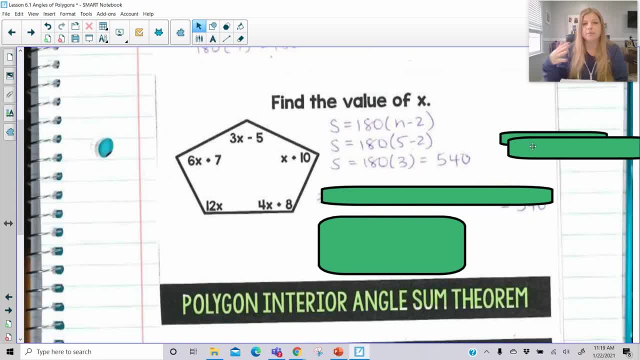 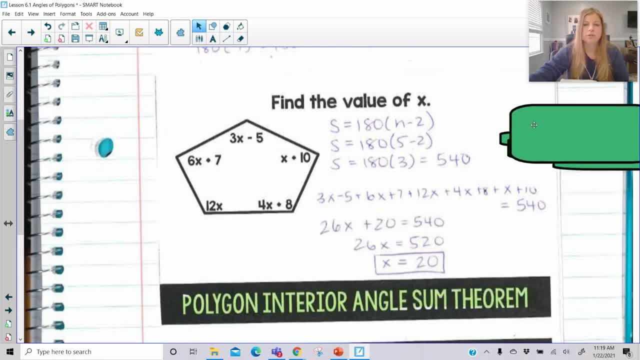 Until I'm able to solve for X and I end up getting X equals 20.. And of course I could go in. I could substitute 20 in for X, add them all up, make sure I get 540. And I know I'm going to be good. 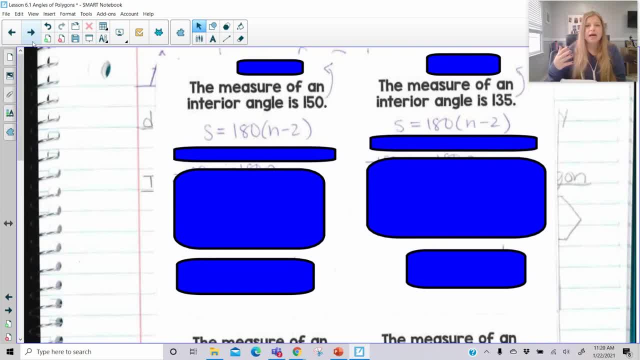 Now, if I was to ask you to figure out how many sides there are of a polygon, if I give you an interior angle. So this is kind of switching gears just a little bit, And so what this is actually saying is the measure of an interior angle is 150.. So what I have to do is I need to 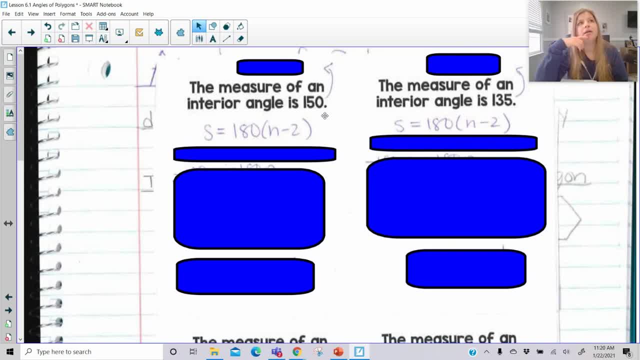 figure out. okay, well, how many sides of a polygon does there need to be? So each interior angle of this regular polygon is 150.. Now the sum, in this case, S, that we were using as the answer before we're actually going to be able to say: okay, well, each interior angle is 150,. 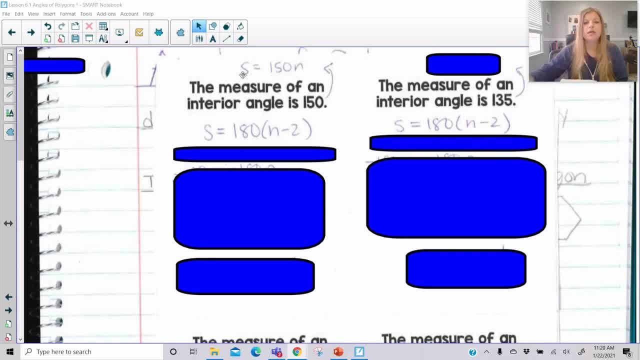 and the number of sides is equal to the number of angles. So I'm actually going to replace the sum of these angles with 150n, So 150n. so 150 degrees times 150n, The number of angles should be equal to 180n minus 360. after I go ahead and I distribute, 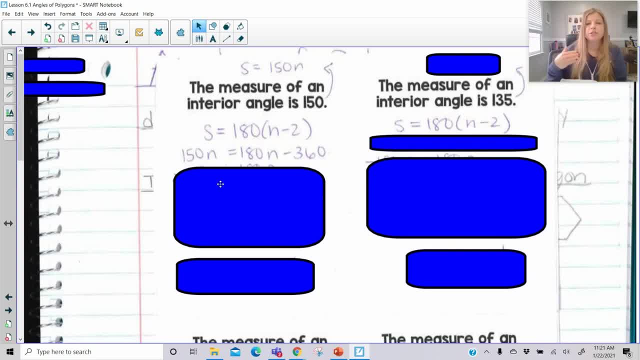 So what we're doing here, guys, is we're not plugging in the number of sides, We're actually solving for the number of sides. We want to know how many sides of a polygon do I need. So each interior angle is 150.. And the S we replace with that 150n, because that represents what the sum. 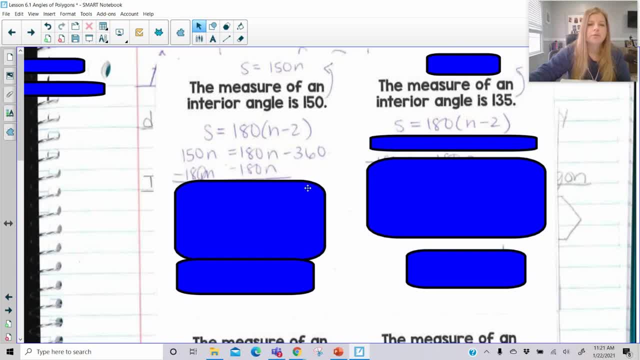 of all the angles is going to be: We're going to subtract 180n on both sides. What you're going to notice here is you're always going to get a negative value. Negative 30n is equal to that negative 360.. But we know we can't have a negative answer which we're not going to. 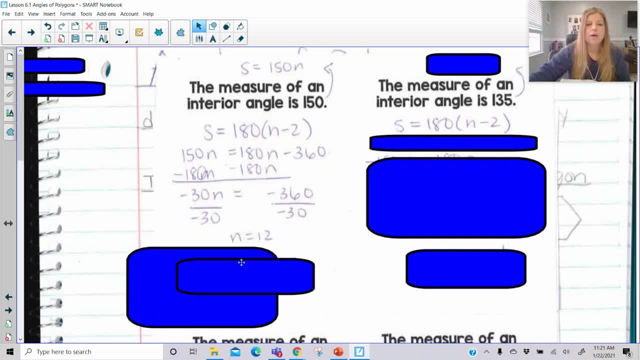 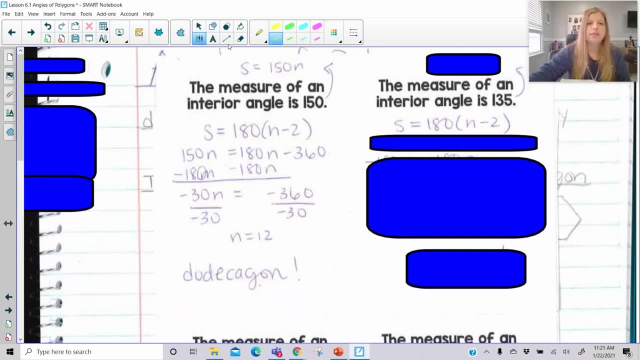 have. We're going to divide both sides by negative 30, and we're going to end up getting n equals 12.. Twelve is a dodecagon. Now to basically put this into writing for you. so if I have a dodecagon, right, So that's 180.. So what does that equal? I have a dodecagon And I have an equal number of dodecagons, right, So I have an equal number of dodecagons And I have an equal number of dodecagons. 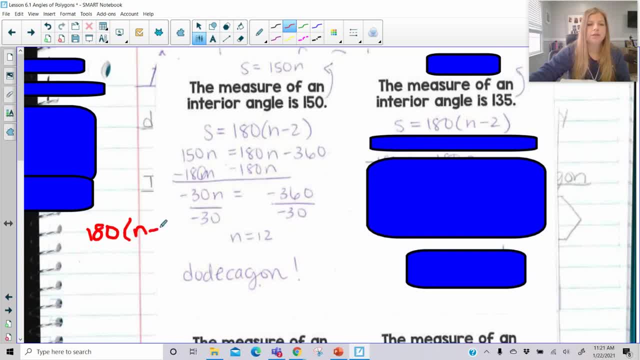 And then if I write this down, I can write 3d. Okay, So if I have a dodecagon right and then I have a dodecagon times n minus 2.. That's my formula, And if I go ahead and plug in a 12,, 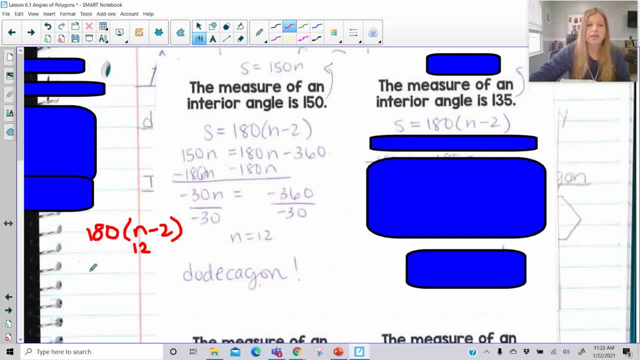 well, 12 minus 2 is 10.. 10 times 180 is 1,800.. So there's 1,800 degrees in all of the angles added up. Now, if I just prove that, it's a dodecagon, think about this. and there's 12 sides if I take. 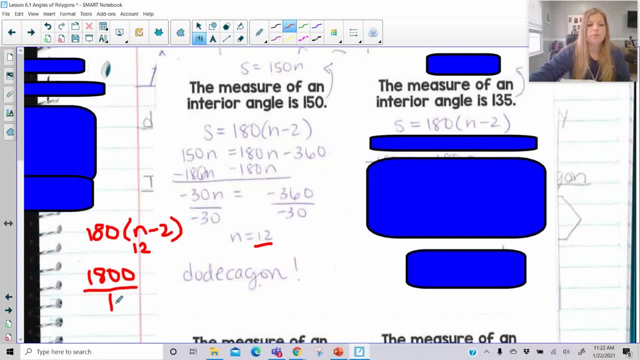 in 12 angles. if I divide 180 by 12 angles, I'm sorry, 1,800 divided by 12, it's going to give me my answer of 150, that each angle is 150 degrees. Let's look at the next one, The measure of an. 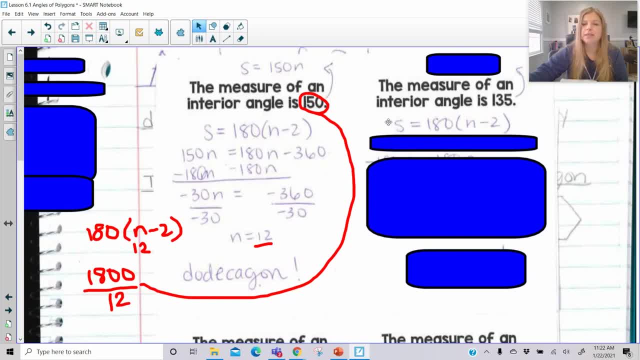 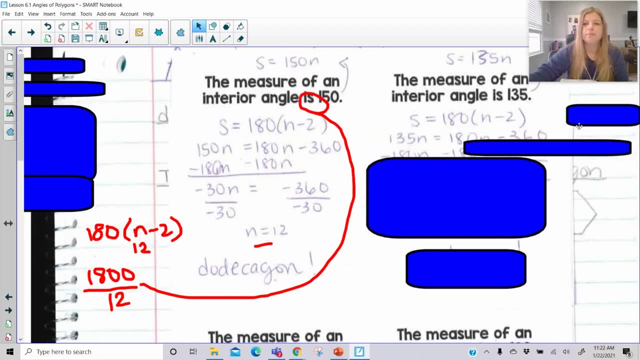 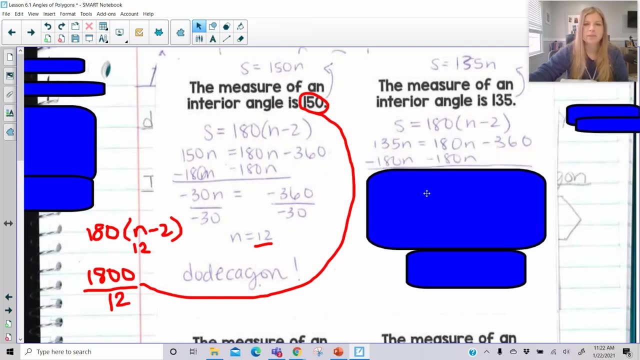 interior angle is 135.. So I'm going to replace the sum of all of the angles with 135n, because it's 135 times however many angles there are. We're then going to continue to just solve for n. So same steps as the previous problem: Subtract. 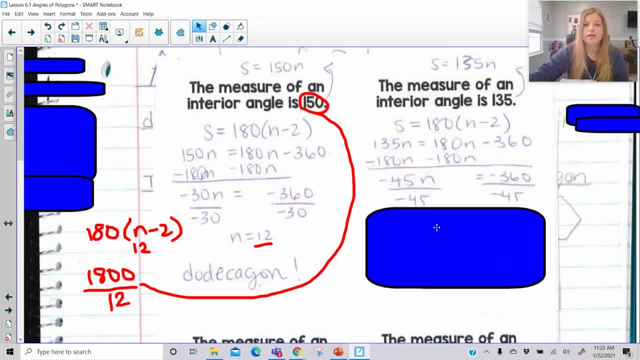 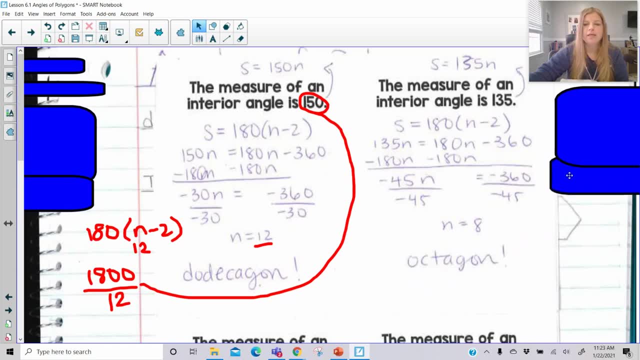 180n, then divide by that negative 45. Always make sure you get a positive answer. We end up getting 8 as the result. We know 8 is an octagon. And again, if I follow the same rules and I went, 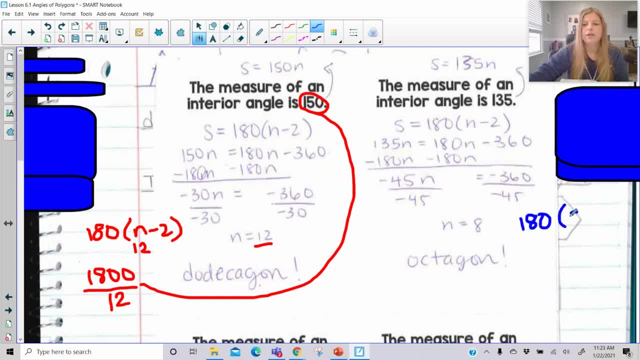 ahead and I did 180, let's see 8-sided figure. so I'm going to do 8 minus 2.. It's really 180 degrees in an octagon. So I'm going to divide that by 8 sides and I'm going to get a positive answer. 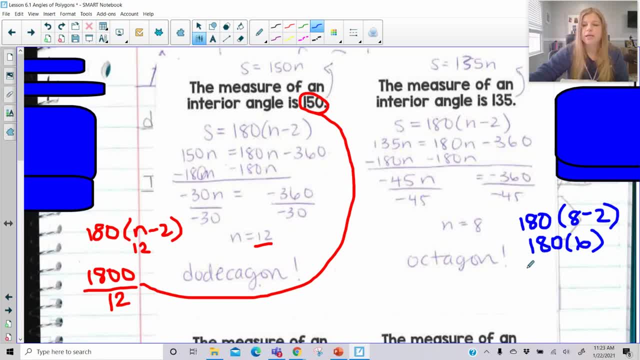 So I'm going to divide that by 8 sides and I'm going to get a positive answer. So I'm going to get a positive answer. So it's 1080.. So there's 1080 degrees in an octagon And if I divide that by 8 sides, it's going to mean that each 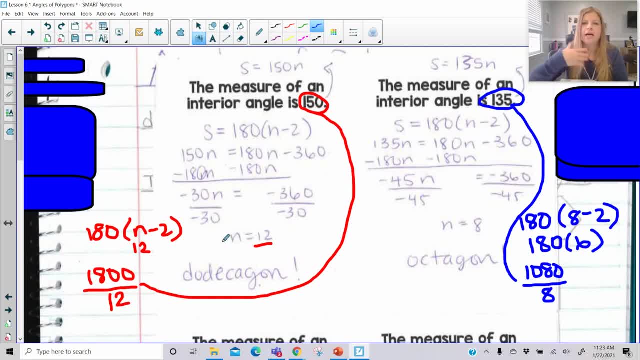 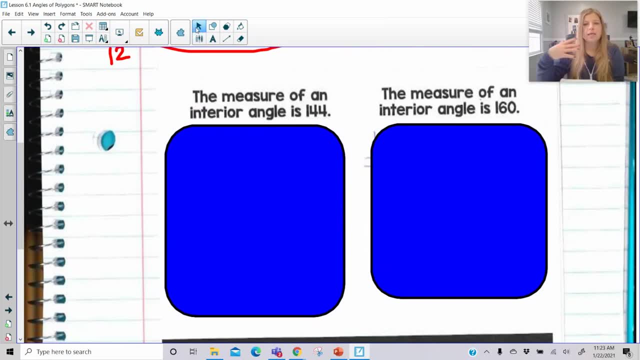 angle is definitely 135.. So that's what we are actually doing when we solve this. These next two, if you want to go ahead and pause and try them out, it's the same process, just different numbers, And then press play when you're ready. 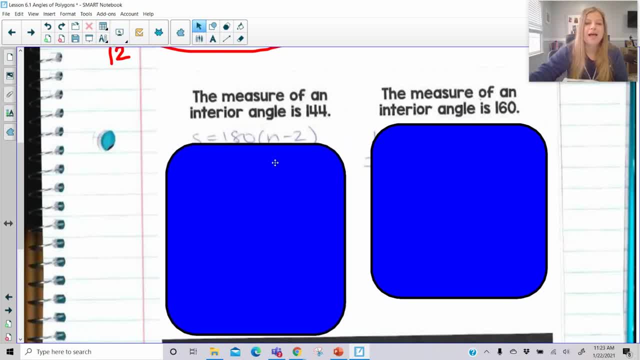 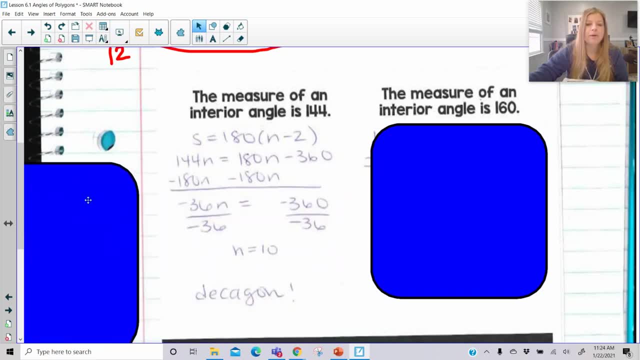 Okay, so I'm going to hope that you pressed play now at this point And you can see what I'm substituting in and how I'm getting my results. That one ends up being a 10-sided figure, which is a decagon. 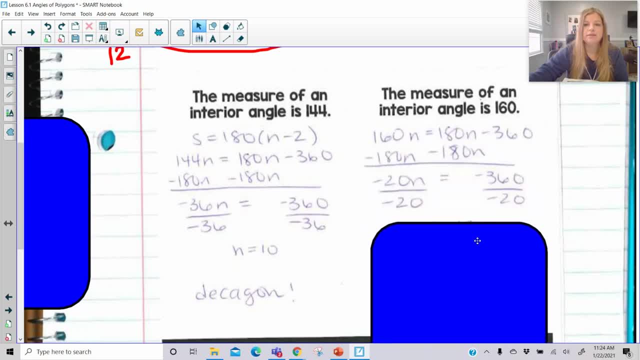 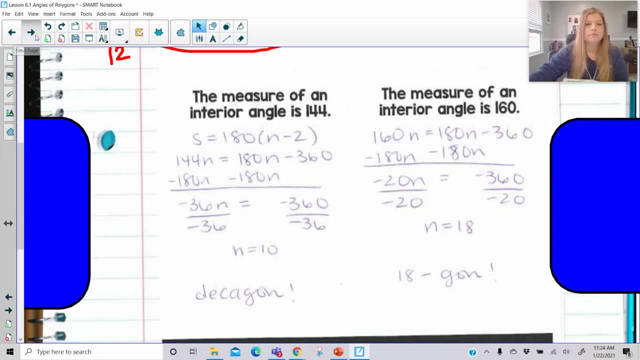 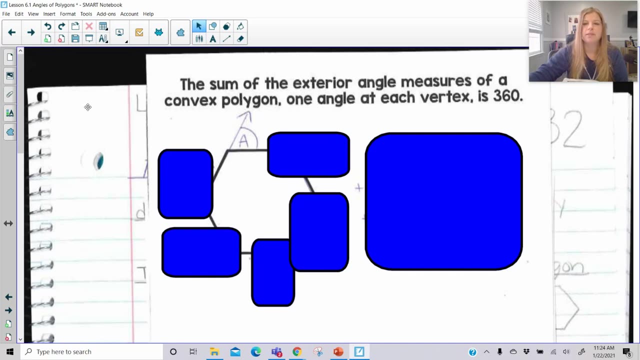 And then, if the interior angle is 160, I end up getting an 18-sided figure, which we just refer to as an 18-gon. Okay, so the last part of this is understanding the exterior angle sum theorem. It says the sum of the exterior angle measures of a convex polygon, one angle at each vertex. 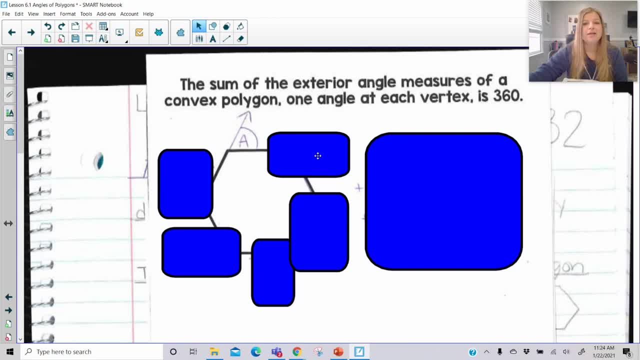 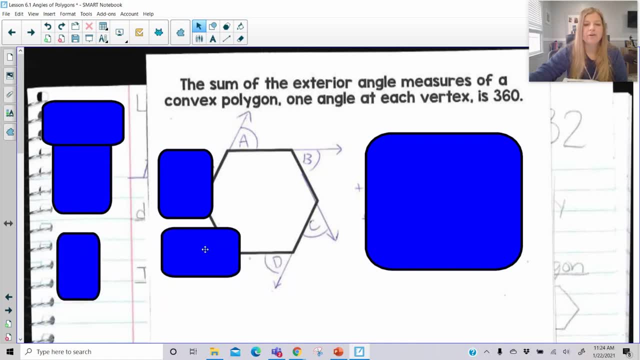 is 360 degrees. This is pretty cool. So what this is saying is if I was to take this hexagon and basically extend the sides of every side of this hexagon and extend it, so I make these exterior angles- they're called exterior because they're on the outside of the polygon- all of these exterior angles. 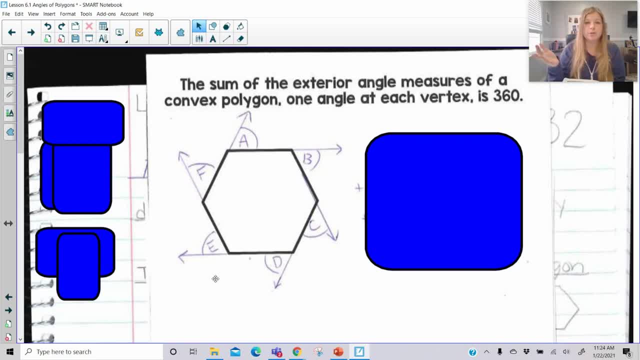 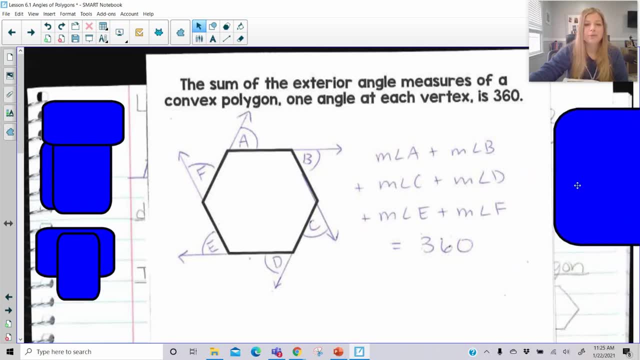 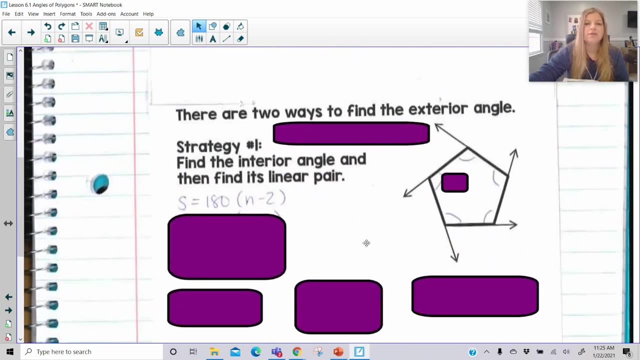 whether it's a hexagon, a pentagon, a quadrilateral, an octagon, a dodecagon is always going to add up to 360 degrees. okay, It is pretty cool. okay, It's always going to be that way, no matter what the figure is. 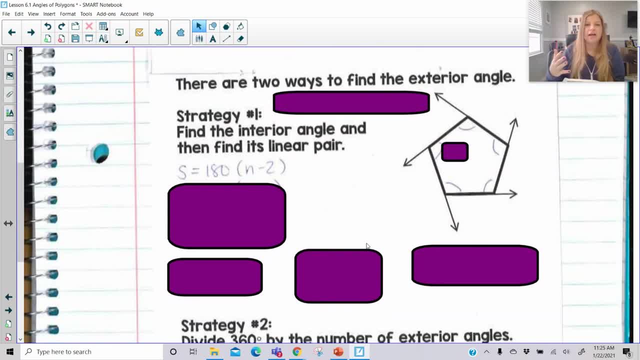 So now, if I said to you, hey, I want you to actually find an exterior angle, there's two strategies for basically trying to figure out the measure of an exterior angle, And this works with, of course, just regular convex polygons. So strategy one is to find the interior angle and then find its linear pair. 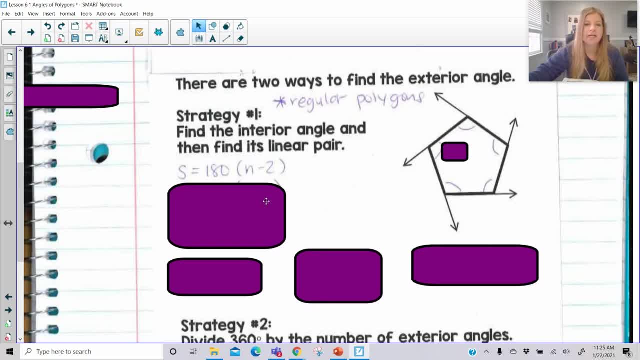 So let's say, in this pentagon I go ahead and I'm like: okay, there's five sides, I'm going to plug in a five for N. I'm going to figure out that. okay, there's 540 degrees in this pentagon.